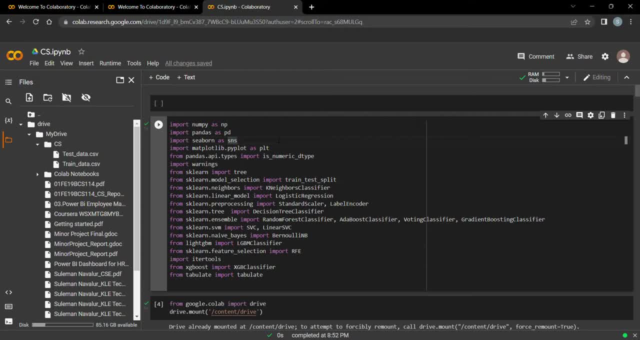 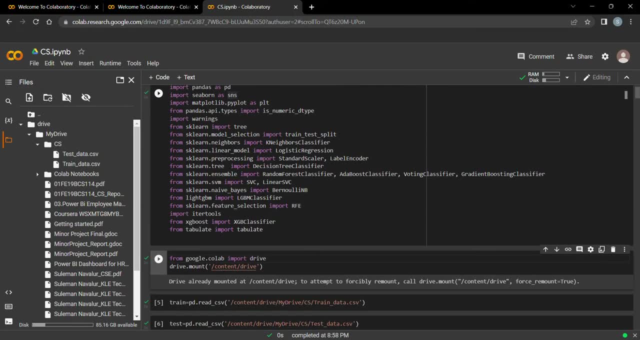 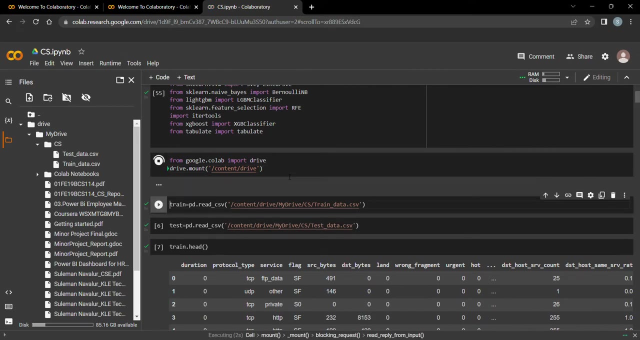 load the libraries, libraries such as NumPy, Panda, Seaborn, Matplotlib and some scikit-learn libraries. So let's load the dataset. So let's mount the drive. So as I upload the dataset in the Google Collapse, so I have uploaded the data in the drive itself. Let's load the. 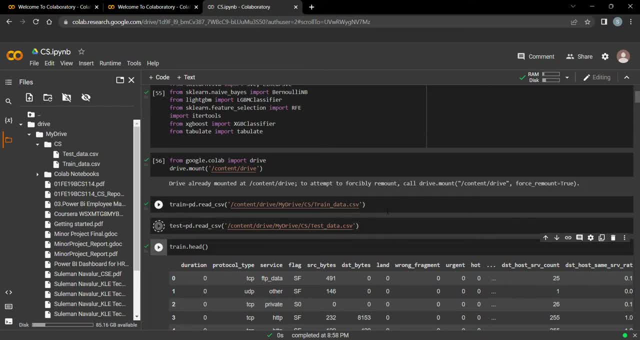 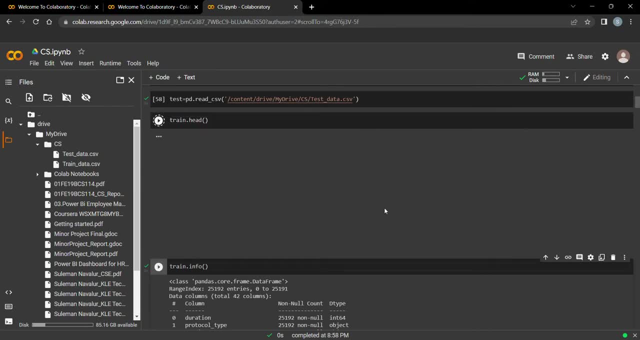 train and test dataset. Let's see the first five records of the train data. So we can see that there are 42 columns, such as duration, prototype service, flag up to distance, destination, service, port and class Class. 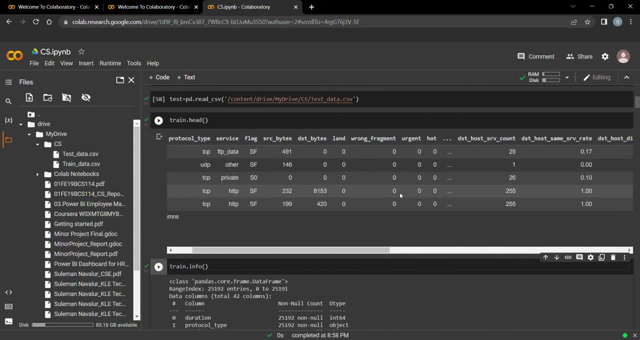 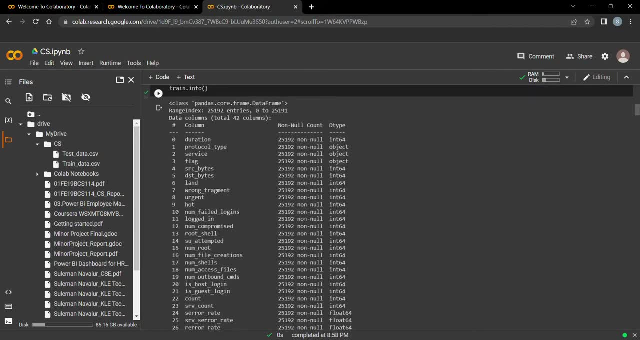 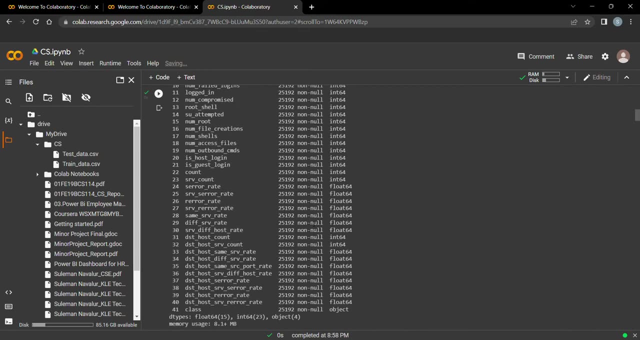 there are two classes- normal and anomaly- for our dataset. So let's get the info of the train data So we can see that there are 42 columns and none of there are none, none, null, So that every column has some data and there are different data types, such as: 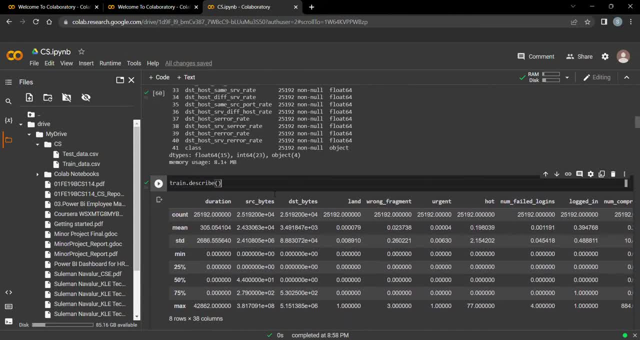 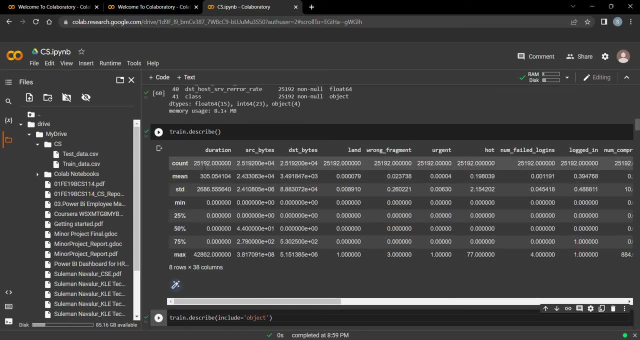 integer and object data and float. Let's just describe the train data. So we can see that there are 24,192 records in the train data with mean of 305, standard deviation: minimum, 25%, 50%, 75% and max. So it describes. 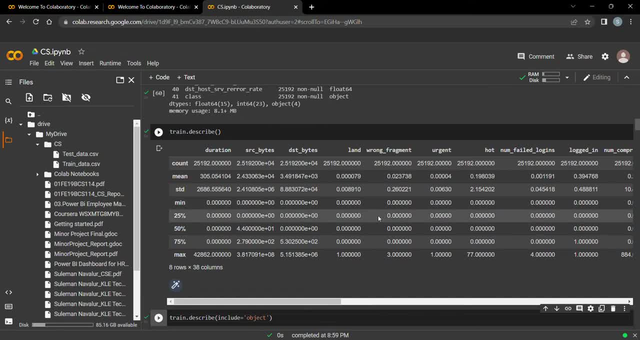 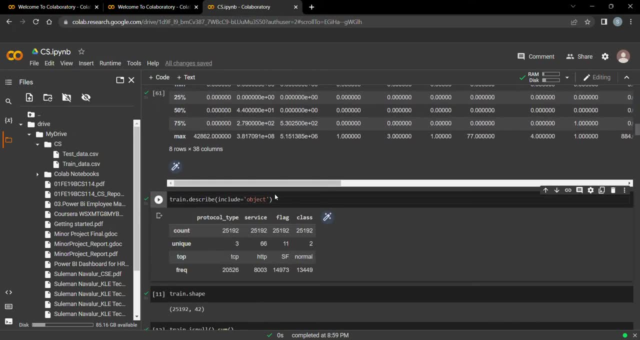 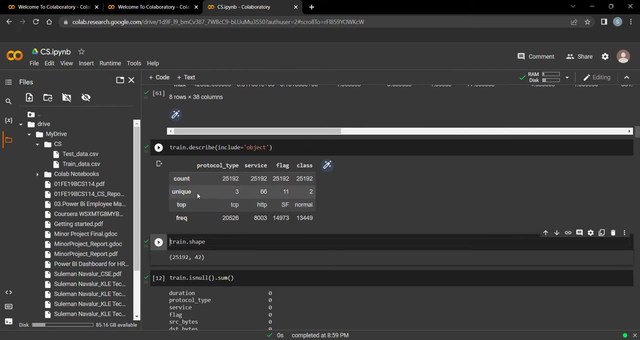 the uh curve count min, max and F for every column. so from this we can describe for 38 columns. let's describe for only object type: data, data type. so from that we can see that there are only three object data, such as unique, top and frequency. so the let's 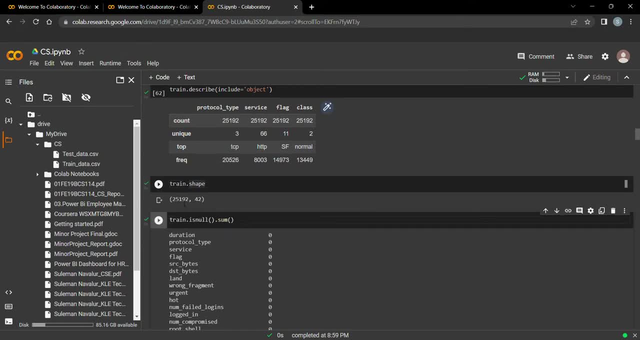 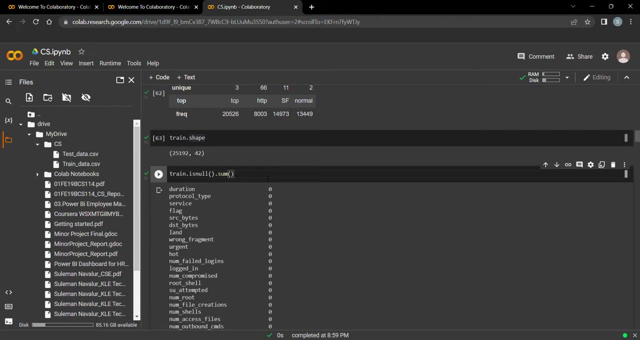 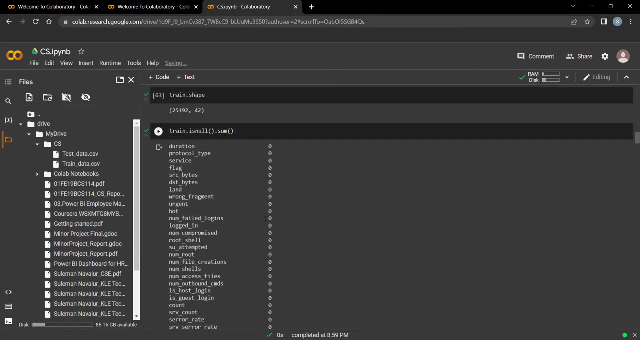 get the shape. so shape is 25,000, 192 records with 42 columns. let's see if there are any null values in our data set and sum them up so you can see that there are no null values in the data set. all 42 columns are showing the sum as. 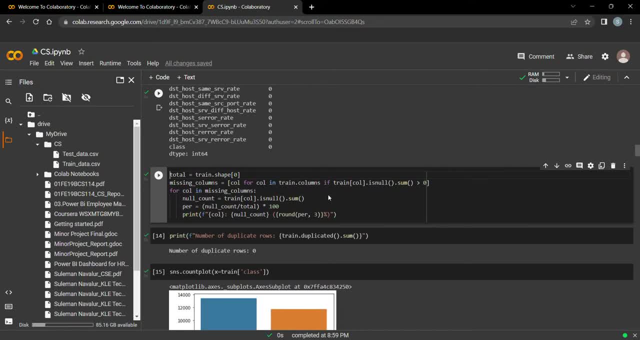 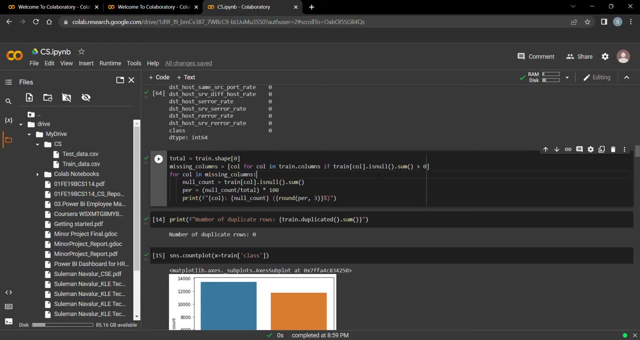 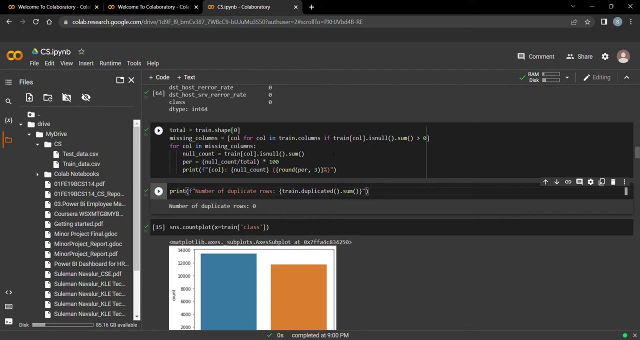 zero, so our data set contains no, none values. let's get some visualizations like how the data set is represented, how the classes are, so let's get a missing data if they're gonna calculate. the missing data case contains some miss columns or null data, so we can see that there are no. 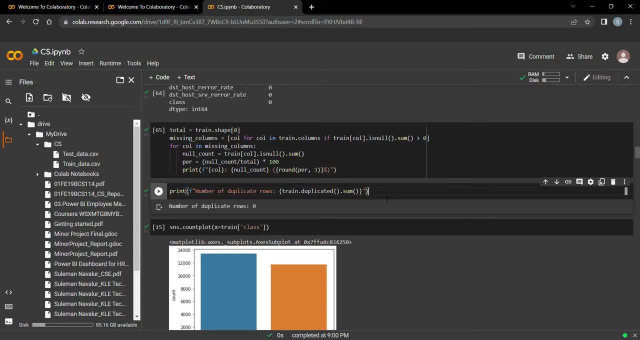 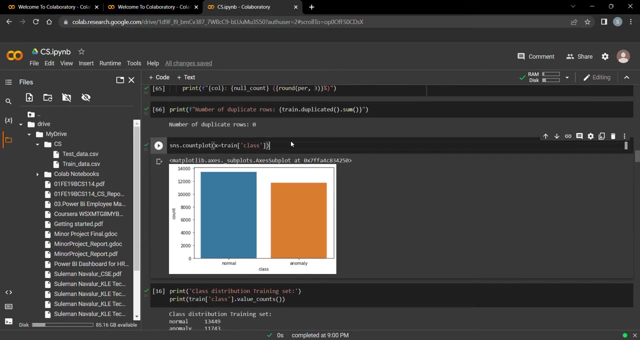 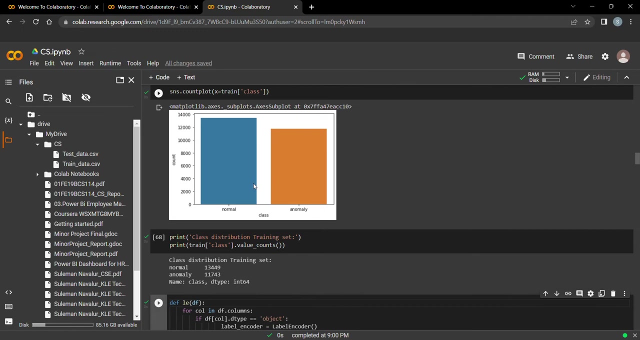 null values or missing value. let's get any duplicate data in our data set so we can see their number of duplicate rows or records are zero, so there are no duplicate values. every record is unique from c1. let's get the count plot of the class. let's get the number values also so we can spawn this crap you can. 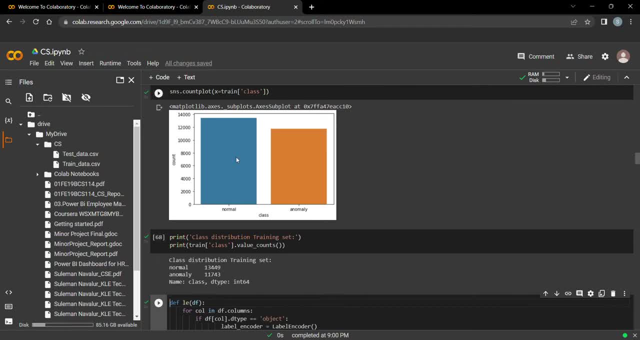 slash that, the noise you will. blue color, the normal has 13,000, one in 14, and courts that are normal, so that the network is normal for what? thirteen thousand records almost, and for the analyst, 11,000 is abnormally like the network is. 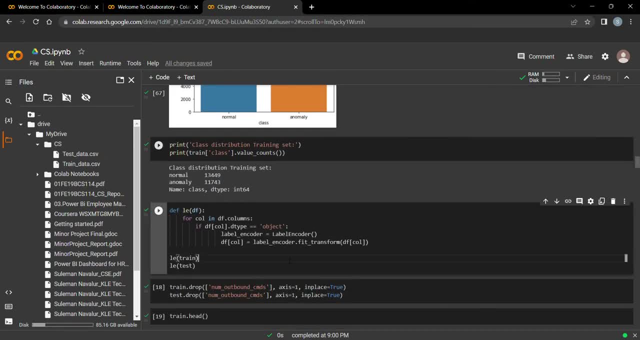 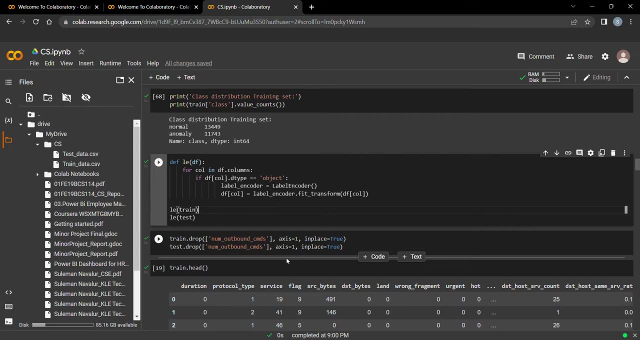 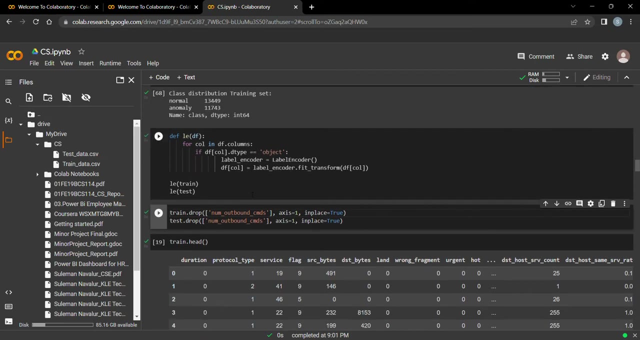 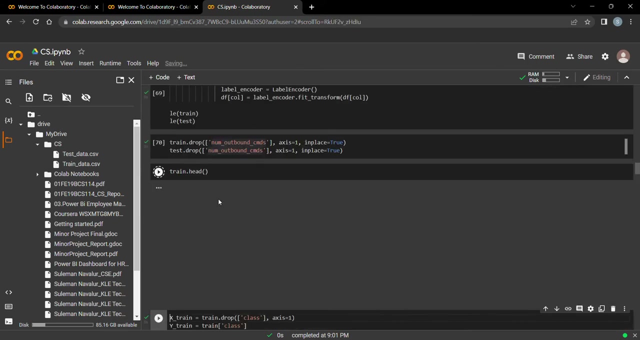 some mean. so detection, like inclusion, is there detected. so let's encode data so we can see that the data has contained some on swing values. so to encode. so I use labor encoder to both train and test the data. so we have encoded the portrayal and test data. let's jump into next part. let's get the train data from this. we 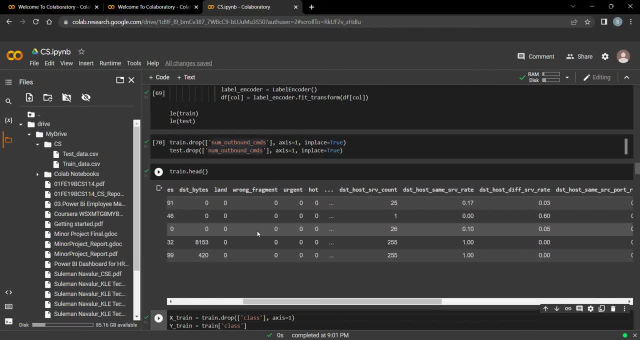 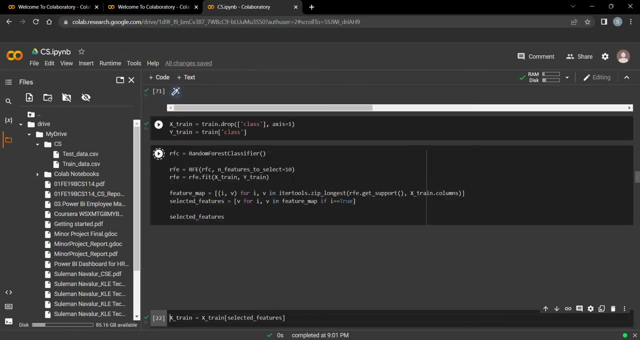 can see that all the columns have categorical values, that is, numerical values class. next step from this random forest class where we are choosing the best selected features. there are 42 columns, so selecting the top 10 column columns or selected features for this, like all 42 columns, may not be used for. 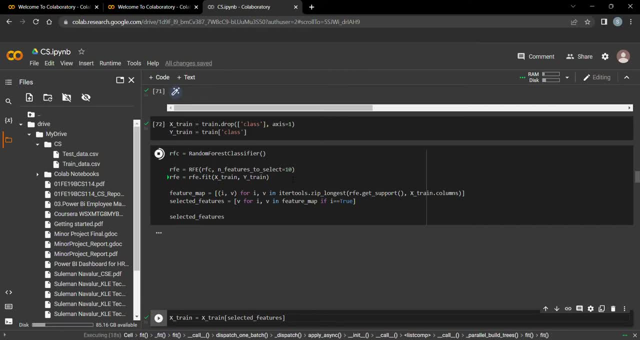 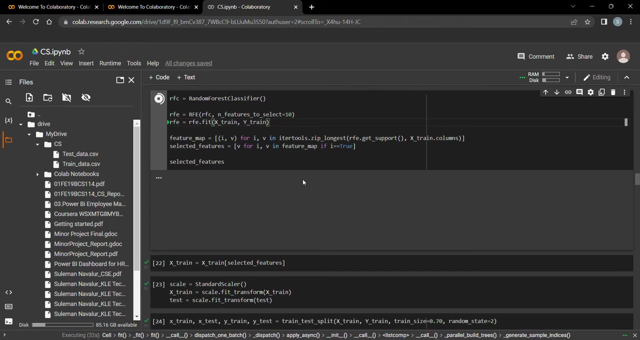 training. so we are using only the top 10, like we have marking the features. that selecting only the top 10 features for our data set it takes time. let's wait for second second. so we got at most the 10 selected feature that our prototype type, prototype service flags source, bytes, destination. 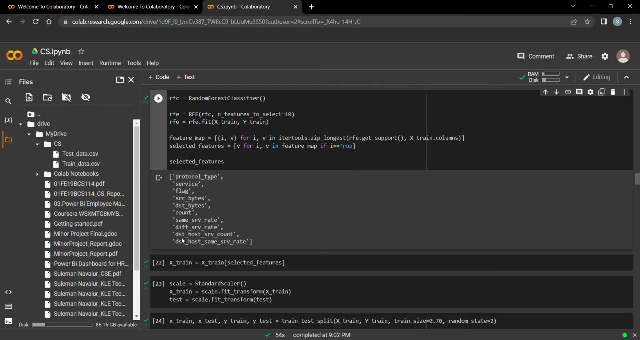 bytes count: same service rate, different service rate. destination would service count decision post: same service rate. so these are the ten selected features from the random forest classifier. so these are the seven selected features for this mix value class am소리. here we can access three rows of filter by default within this. 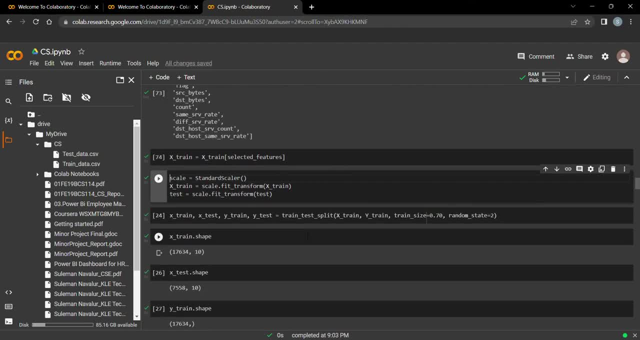 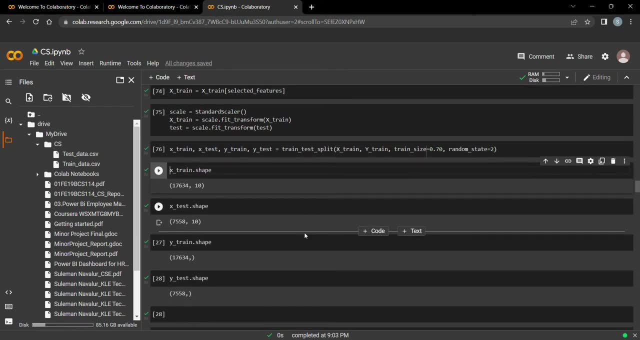 right column am: accelerate through the Redнд3 plugin. then, once again, we will get the. let's get the train data for the selected features. let's get the report train and test both. let's get the shape of this, uh, this 10 selected features. now, this has lifted the data in 70s to 30 ratio, so from this you can see that there are 17. 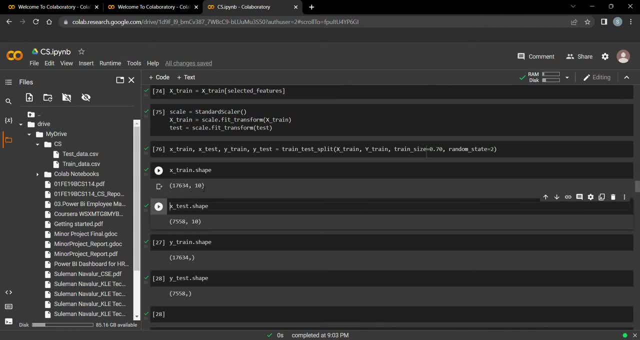 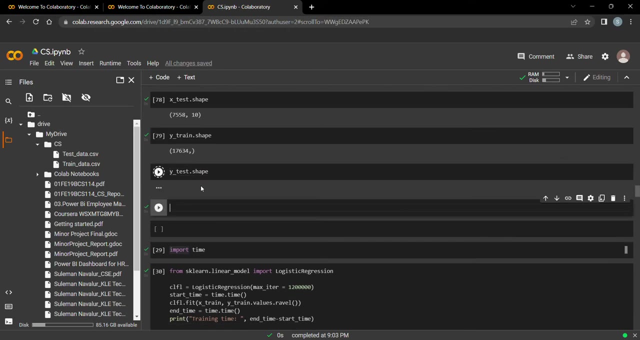 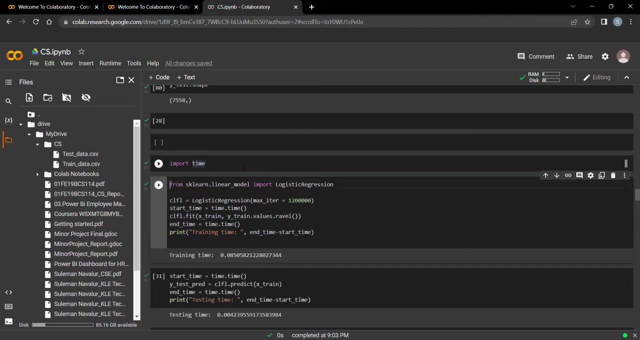 634 records, 10 columns right, 10 selected features for the train data, and so for test data, there are 75, 7558 with 10 selected features, same for training test. let's import the time, like how much time each model takes. so basically, uh, we have used three models that are logistic regression, uh, knn knes, neighbor and 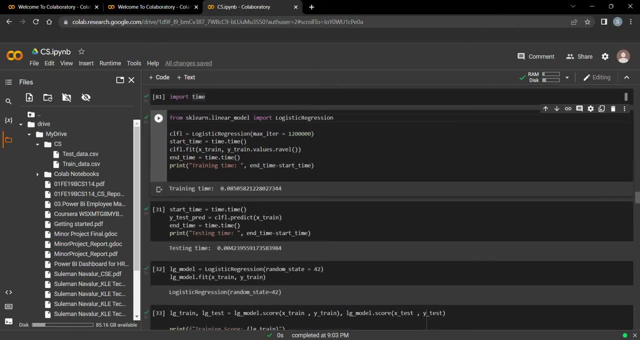 decision tree. uh, let's get to our first model, that is, logistic regression. so for logistic regression we have max taken, max of almost one lakh iterations for the tasks, time taken for each time taken to or for this 12 lakh uh iteration is 0.09 seconds. 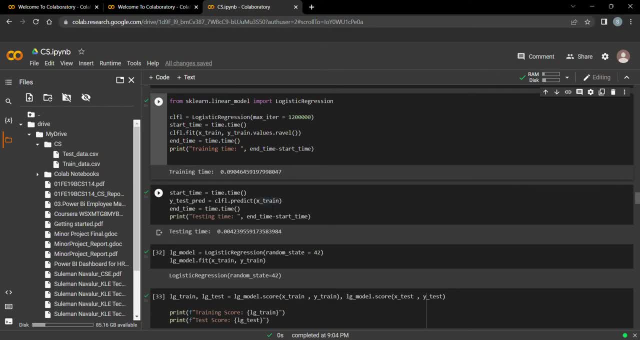 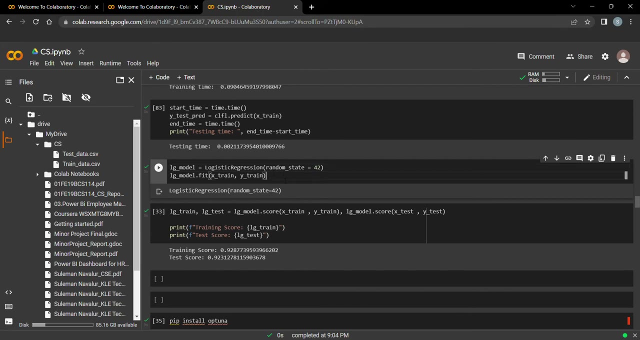 so me it's really awesome. it's taking some more time for it's for train data. let's get for the test data. say for logistic regression model, the test test timing is point zero zero two seconds. ah, it is taking less time. so let's get this to random state, for this allows degradation. 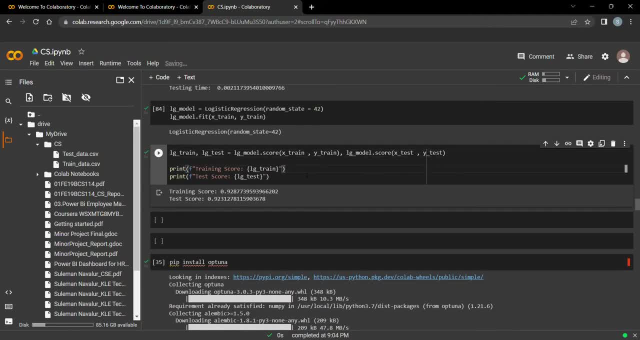 that is 42 random state. now let's get the fit the model. let's get training and test score. for the logistic regression model, we get the train test score as uh 9.92. this is 92 percent accuracy or test score we have got for a large regression model. uh, let's get. uh, let's some other libraries. 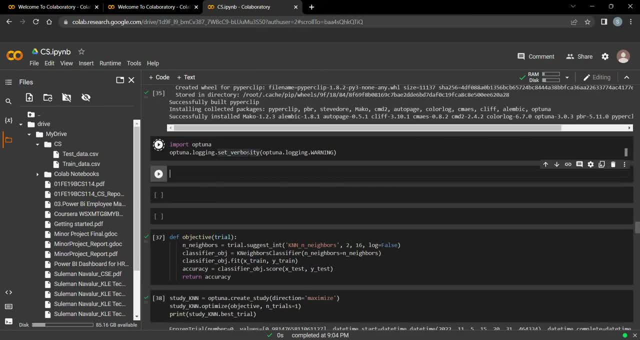 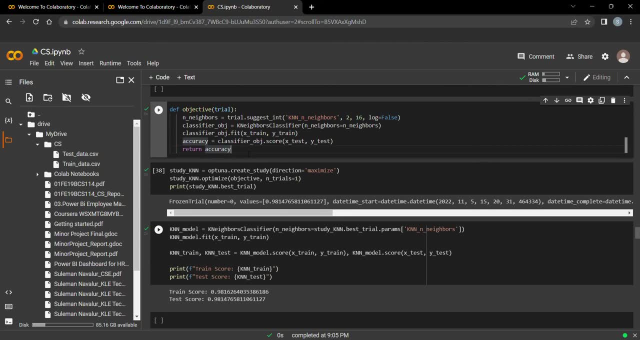 for the next uh model i imported up to now. this is an uh hyper parameter framework. uh, now our next model is uh knn knes neighbor. so for knn, what does it do? is uh? there are two classes in our data set, like in there are normal and anomaly. so based on the features, it groups. 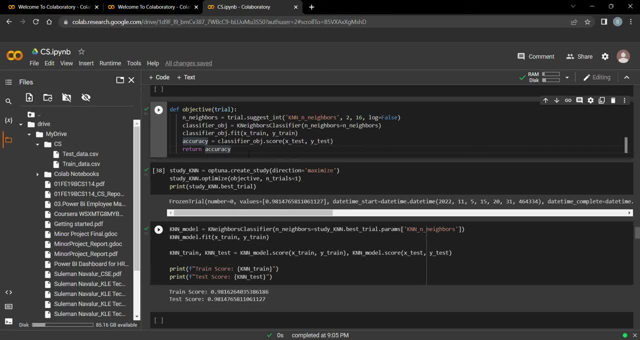 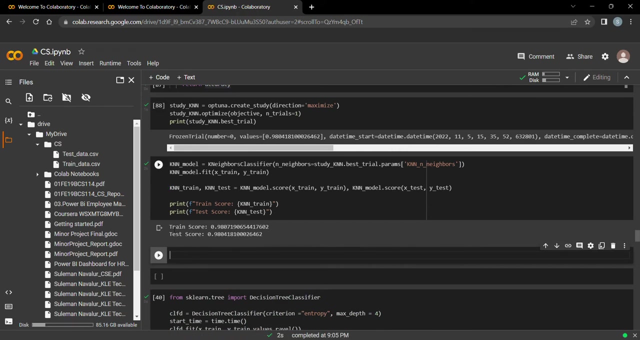 clusters, uh, the two uh similar, similar records to that. those two clusters like: uh, some cluster having normal records and another cluster having anomaly records. let's run this. let's get the training test score for knn, model ah, so you can use a higher code. then high test and train score for knn, greater than logistic regression, is 0.98 across 98 percent. 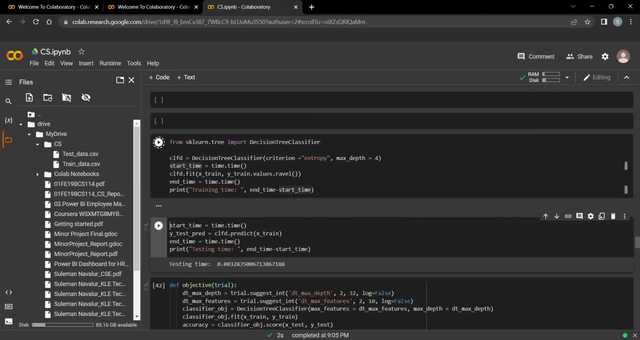 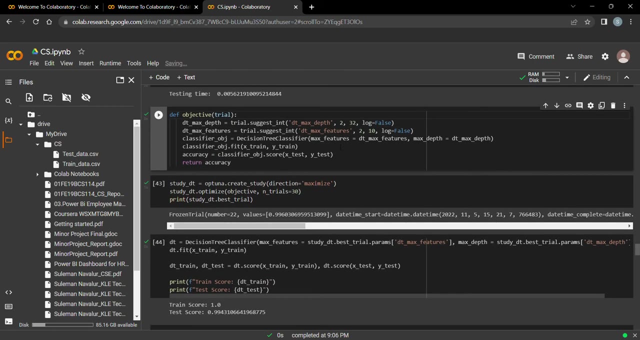 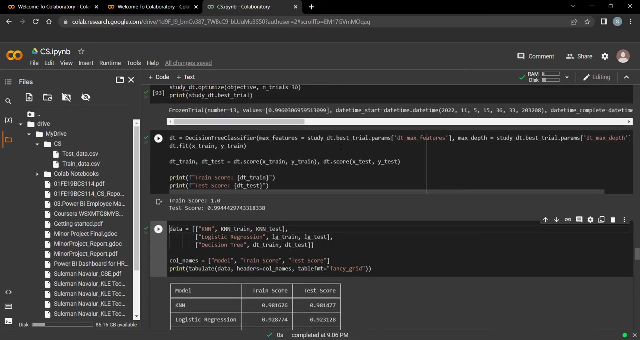 so let's get to a third model, that is, decision tree. decision tree: what, uh, the time taken is is 0.02 seconds and say for the test data it's 0.005. let's pick the model. uh, so let's get the train and test score for the decision tree. ah, so we can say that the try test. 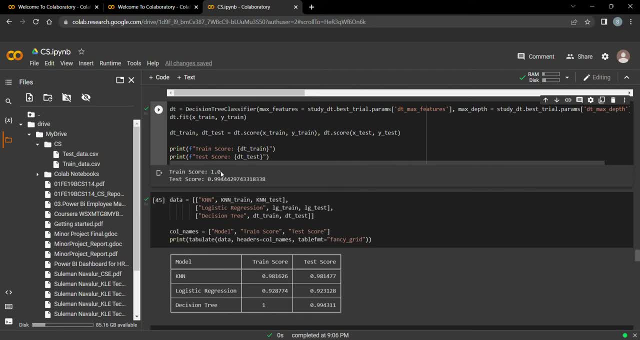 score for decision tree is 34, train is one like is 100 percent and for the score is 0.9, and so decision is performing better than logistic regression and knn. so decision tree is performing better. okay, log knn carry is better for following than logistic regression. let's get the summary of. 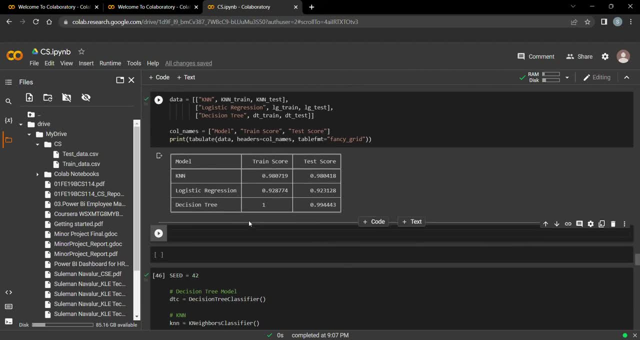 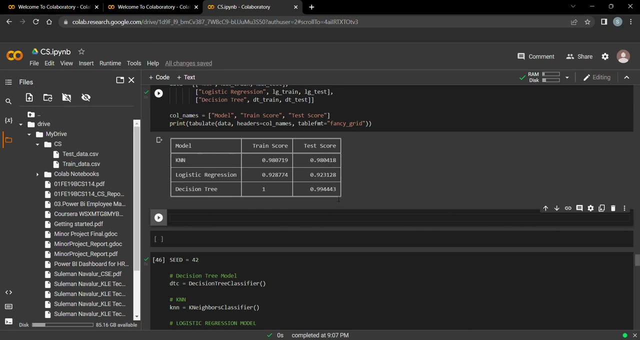 the train underscore. from this we can see that logistic regression, uh knn, is having a trend and test score of 0.98 with logistic regression, 0.92. with decision tree the highest is the point if this is 1 and 0.99. so decision tree is the best model for optimal for intrusion detection system. 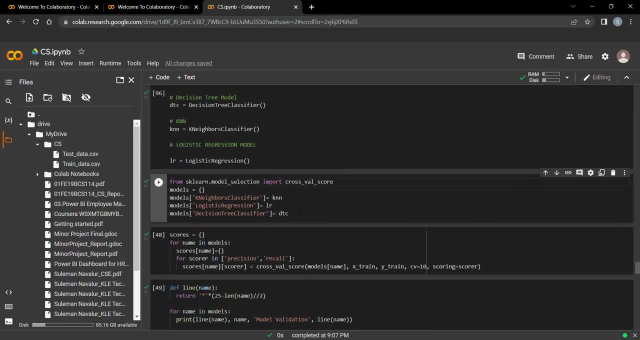 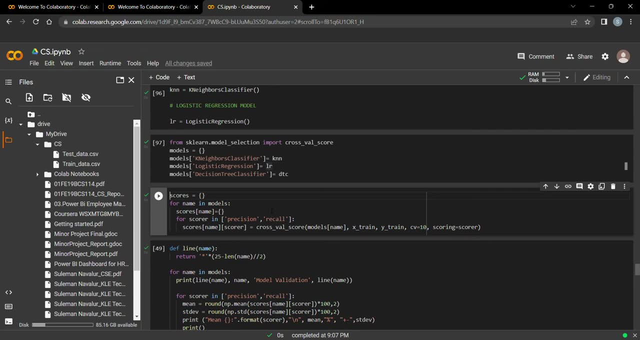 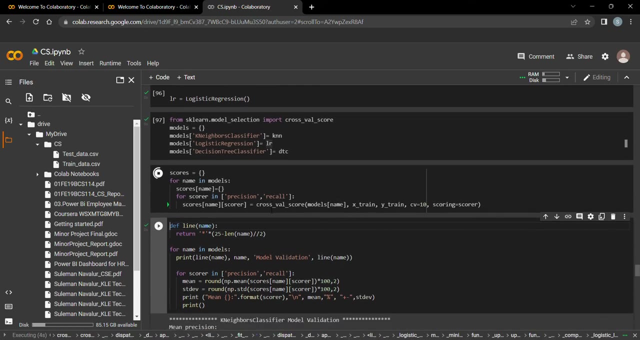 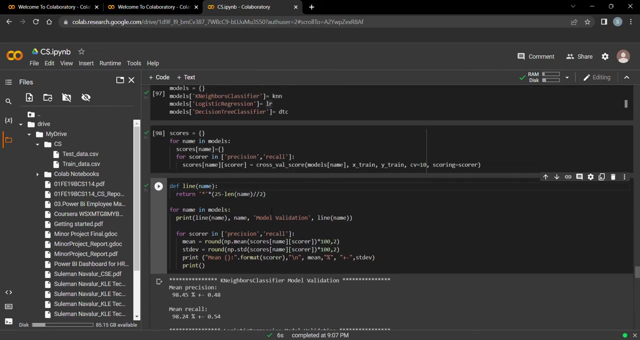 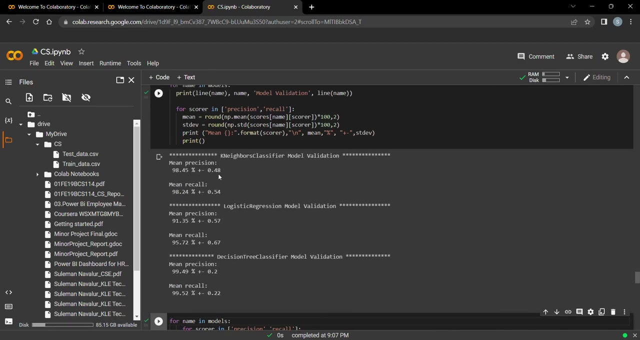 let's get some other visualizations for this training test course. so the testing, the data, let's- uh, let's test the data for other like data. for the test data, let's calculate the precision recall for this. uh, with three models. it is logistic, regression, knn and decision tree. so mean precision is the point minus 0.48, that is approximately. 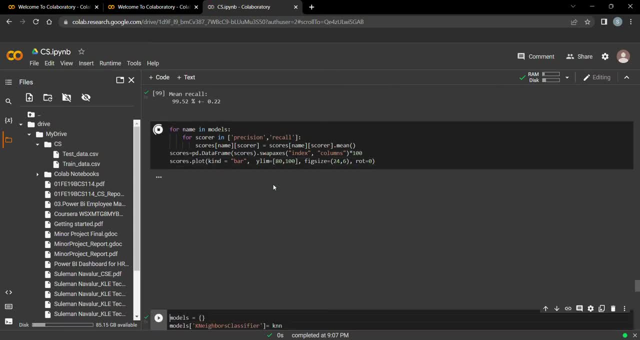 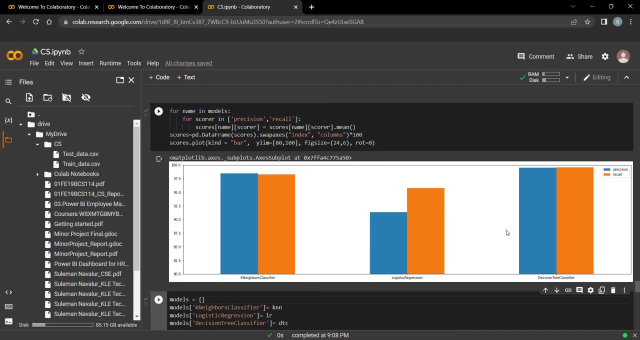 let's get the visualization so we can understand it clearly, so we can see that the decision tree has both, uh the precision recall equal. so we can see that the decision is predicting uh character cost like it, uh it creating the true values. so the in logistic regression we can see that there are some precision is slightly less. 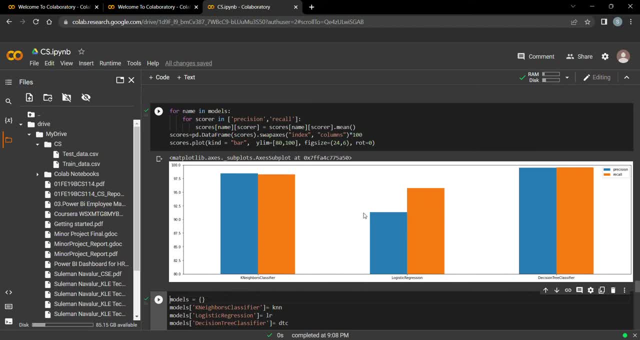 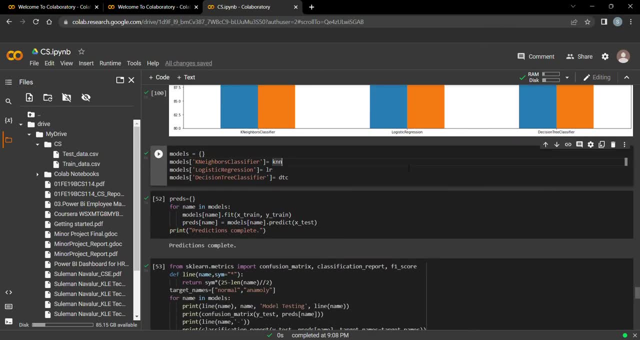 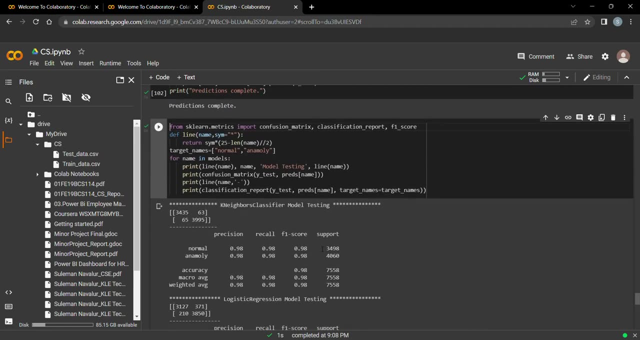 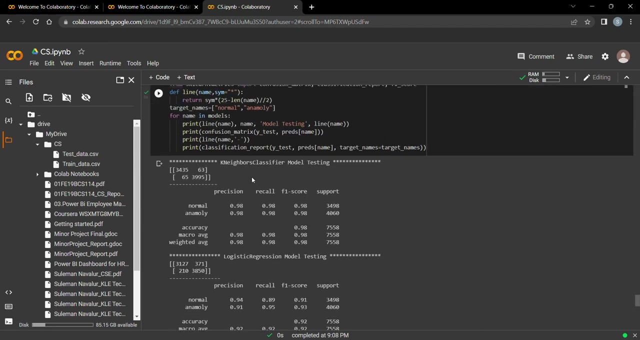 than both the knn and the decision on century and law. the knn is performing good but is not as good as lower decision tree. let's get further intuitions for this. so you have to test the data. predictions are complete. let's get the final precision and uh, recall for this: uh, three models. so for the first model is: 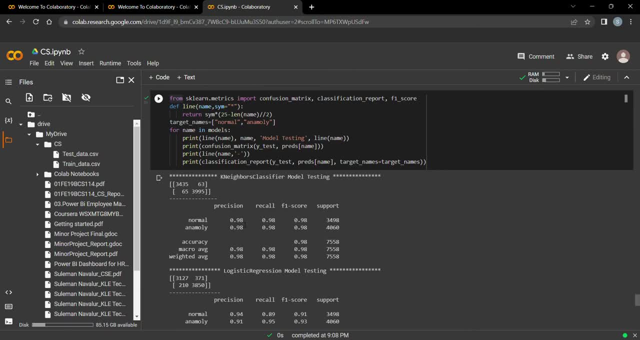 knn. so we can see that uh, precision it normal is 0.9 and recall is 0.9, difference is 0.9. so there are 3035 true positive data values and the true negative is 60.9. so it's slight means some 63 values are not created in true positive. it's not. 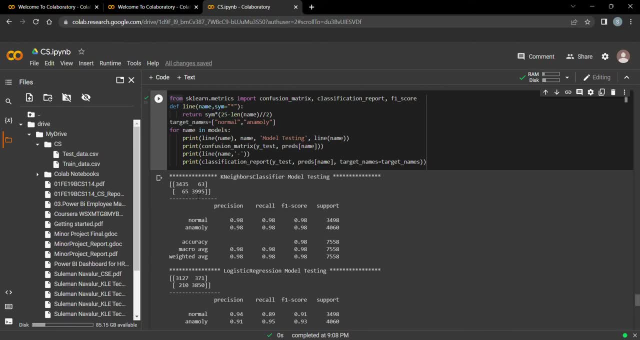 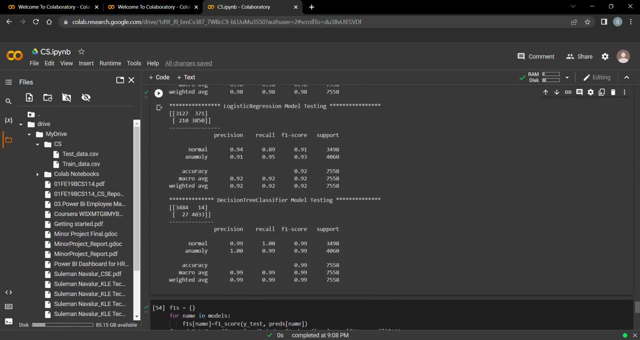 creating is creating false and 65 values are having creating wrong class. in KNN and for logistic regression is pure. the true positive values are 3127 but the true negative values are 300. so it's higher than the KNN, but so you can form.